designing board games, I always wanted to make sure that they were as beautiful as possible, So I decided to make a board game that was as beautiful as possible. and I decided to make a board game that was as beautiful as possible. and I decided to make a board game that was as beautiful as possible. 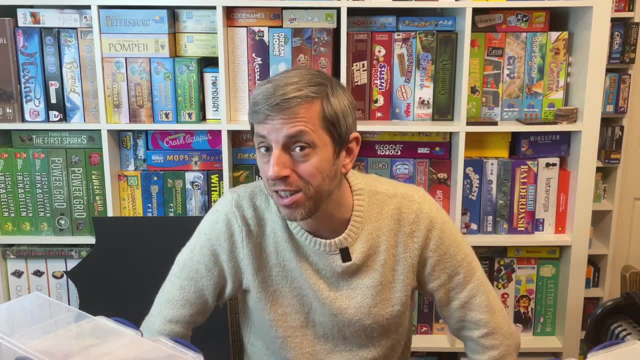 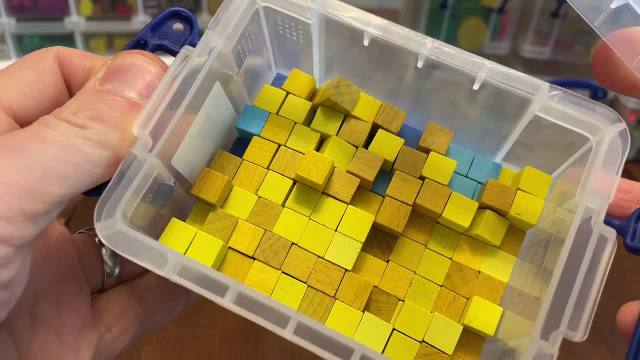 I bought loads of them, but they're surprisingly expensive. One of my first prototypes contained around 100 of them. Checking the Board Game Extras website in the UK just now, they cost 9 pence per cube, so that's £9 per prototype before I even started looking at cards. 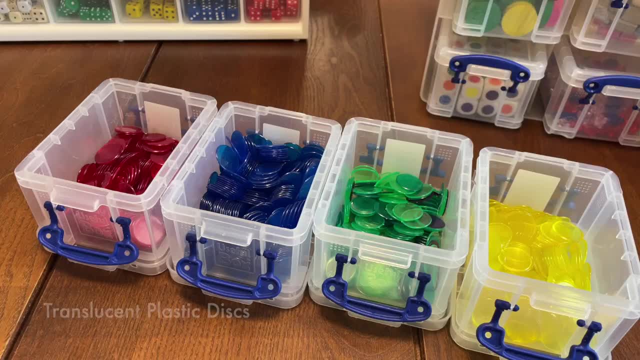 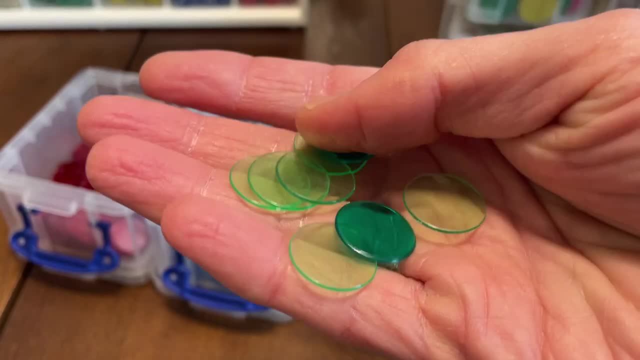 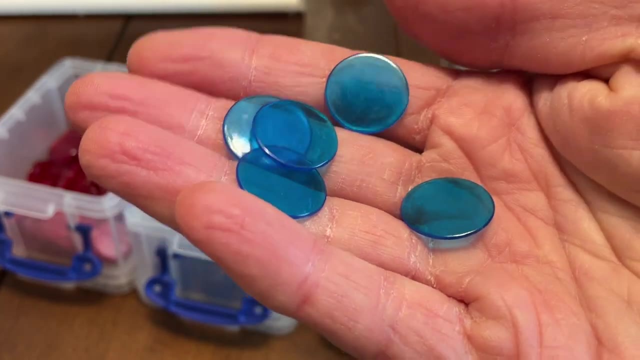 tiles or other tokens. So what's the alternative? Well, one cheap alternative is translucent plastic discs. Currently on Amazon, these are just under £9 for 300, a third of the price of cubes. Colours are a bit more limited, of course, but they're great for representing coins or scoring tokens. 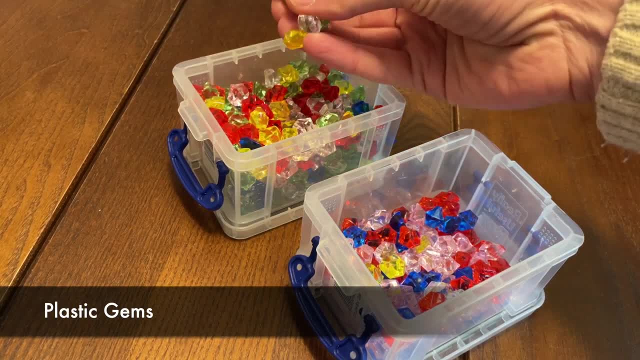 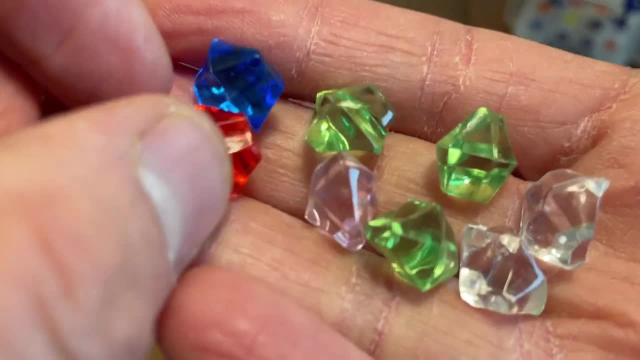 Another option which I love is coloured plastic gems. On Amazon these are currently £8.99 for 270 gems, so they're marginally more expensive than the discs, but considerably cheaper than cubes and far prettier and more tactile. Of course, it depends on your theme. 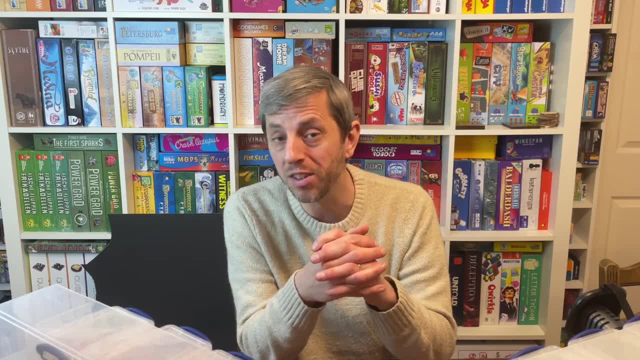 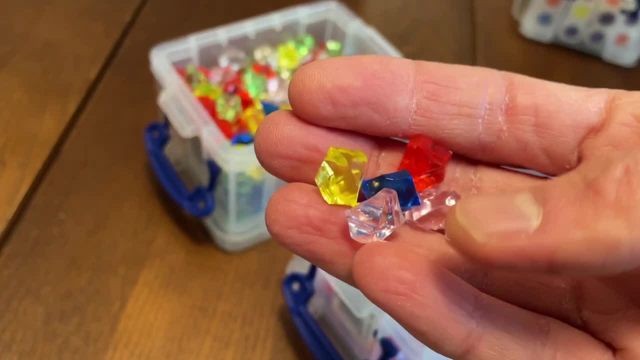 A cube could stand for anything. I struggle to see a gem as anything other than, well, a gem, But perhaps I need to be more imaginative. These are often a gift from stores which sell aquariums. Here are some similar but smaller. 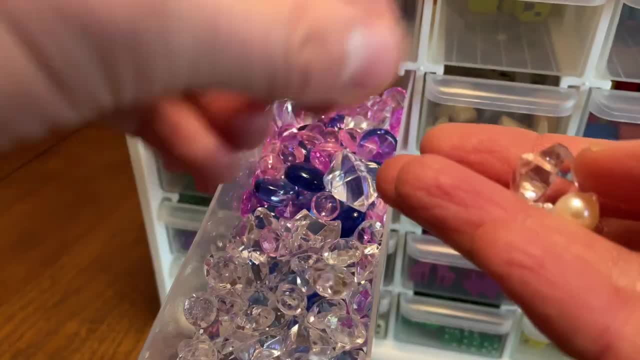 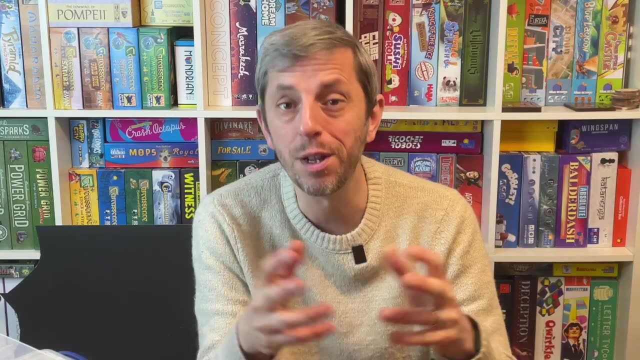 clear gems which my wife has received among the packaging for various Christmas and birthday gifts over the years. I've collected them up for a second life in some future board game. You'll have noticed at this point that I have little units for my prototype components. 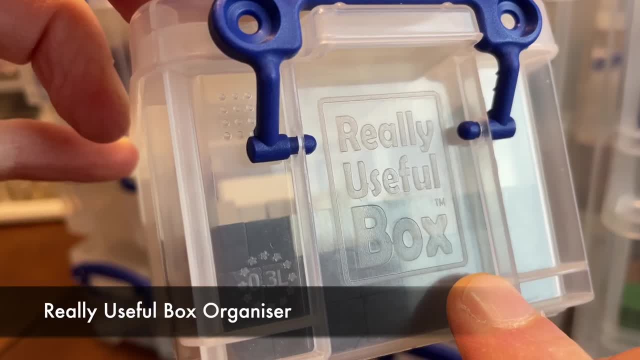 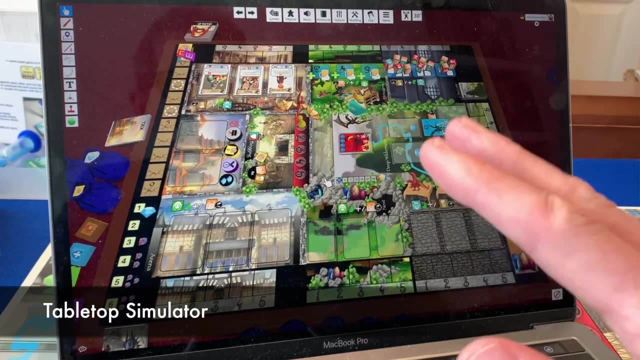 This one came from Hobbycraft in the UK and it's called a really useful boxes organiser. They're not super expensive but they do keep things nice and tidy. Of course, many designers have started to experiment with Tabletop Simulator or other similar platforms to make digital 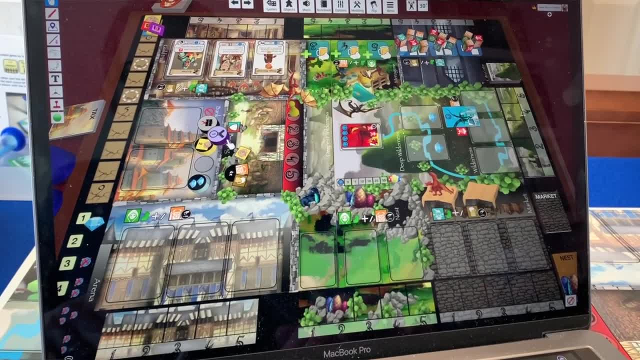 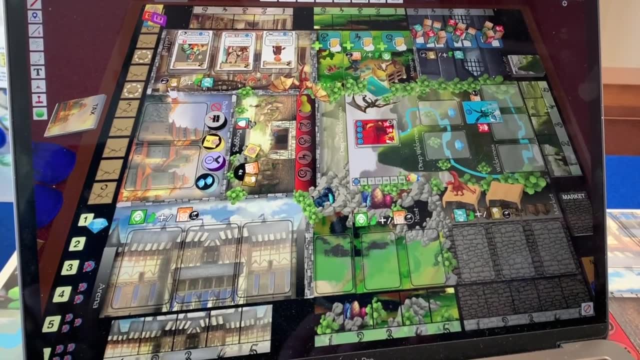 prototypes which can be easily shared around the globe with no financial investment required. I've dabbled with Tabletop Simulator myself, but I'm not going to discuss it any further in this video because, frankly, I dislike using the clunky interface and I'd always prefer wherever. 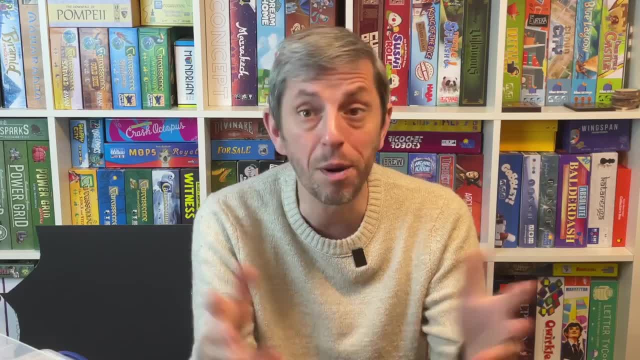 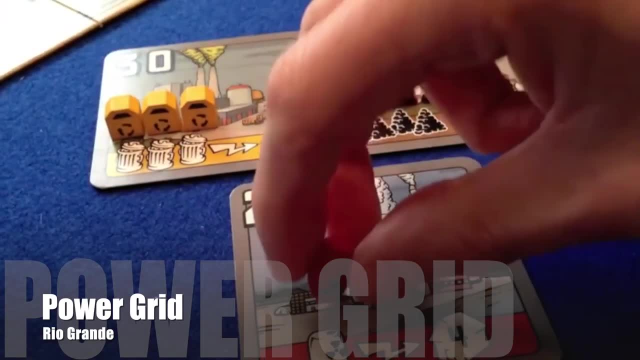 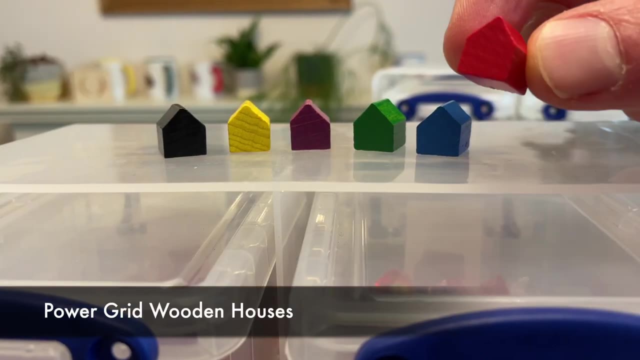 possible to work with a physical prototype With my favourite games. I'm a sucker for upgraded components. Occasionally I'll purchase nice wooden tokens from companies like Meeplesauce to replace the original components, and the original pieces find their way into my box of prototype pieces. These can be really useful for future projects. 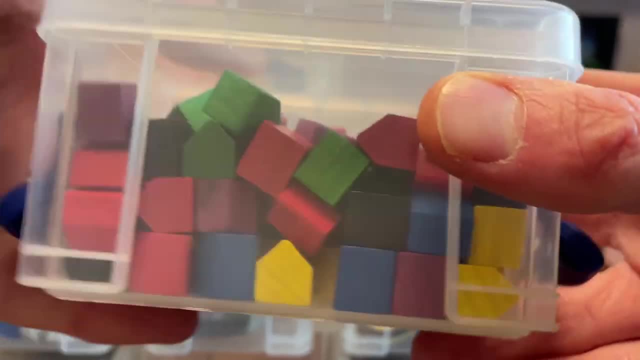 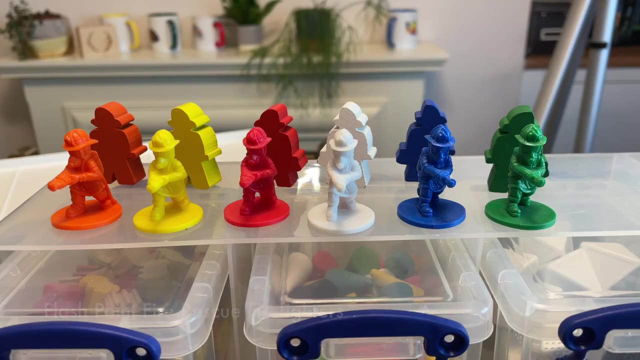 especially if the pieces are very generic, like the coloured houses from Power Grid or the wooden cones from Dominant Species. It's less helpful when the components are unique, like the firefighters from Flashpoint Fire Rescue. Now, I've upgraded this game more than once. 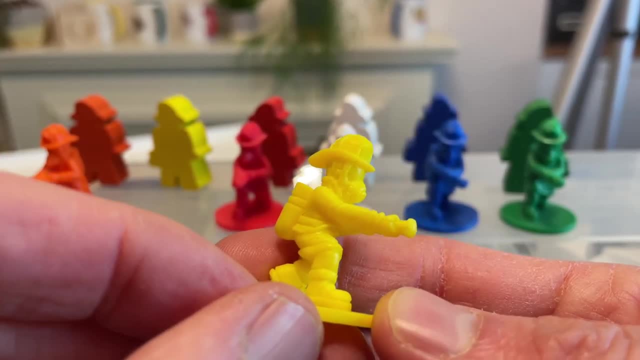 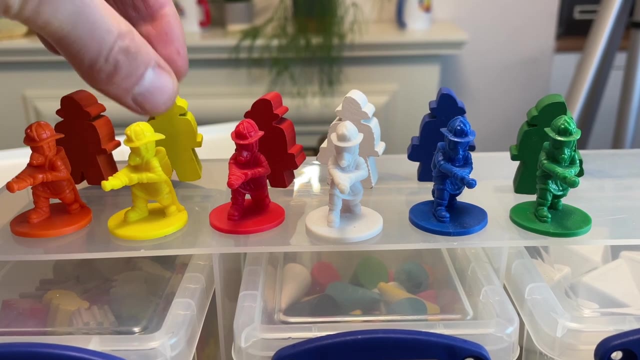 and the firefighters left behind would be great for another firefighting game, should I choose to make one. but the problem is that for any of my projects I'd always need to make multiple copies to give to multiple publishers. so one set of firefighters isn't going to cut it. Nonetheless, 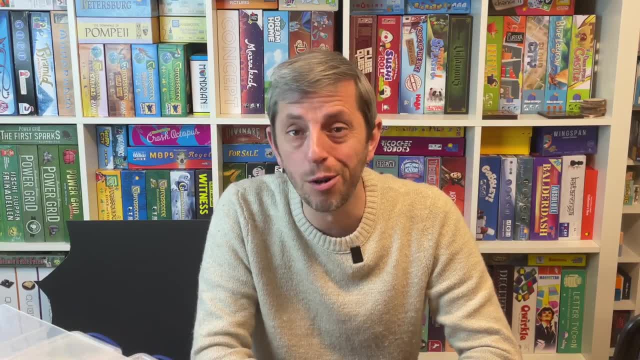 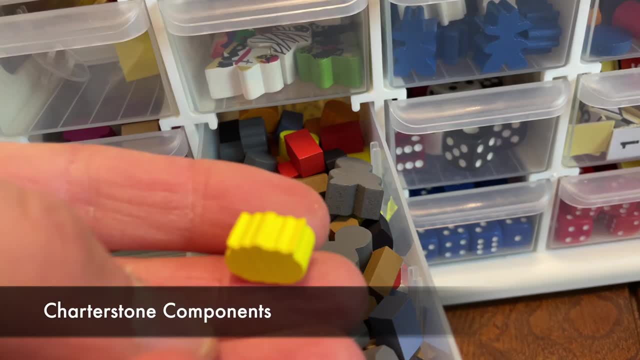 I keep them for inspiration. One game which presented me with loads of great components was Stonemaier's legacy game, Charterstone. It was a really enjoyable game, but once my wife and I had finished the campaign, I couldn't see us playing with the altered board again. 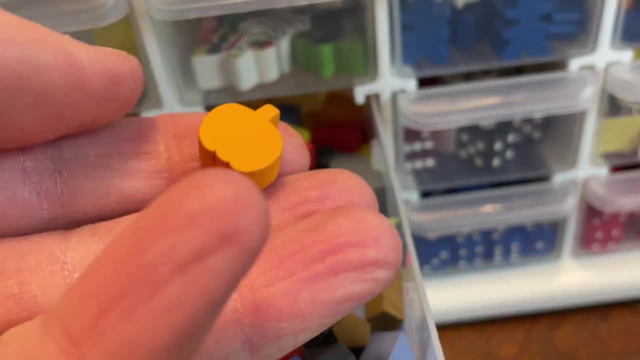 and it was just a big old box to sit on the shelf. So I stripped out the components for my game and put them back in the box, and then I put them back in the box, and then I put them back in the box. 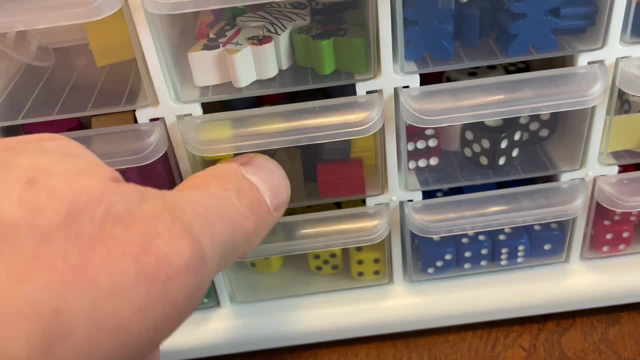 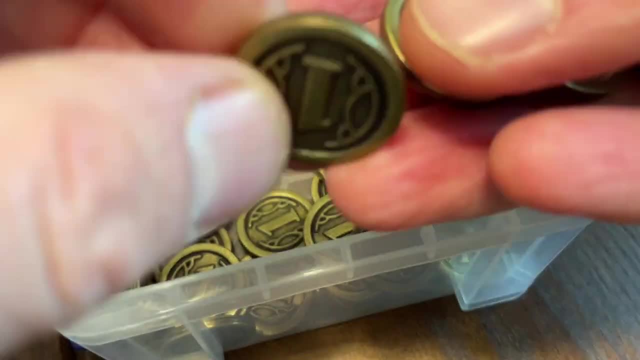 and there are some lovely pieces in there, not least the hefty metal coins. Frankly, I can't ever see me using these in a prototype. Why waste them when I could use transparent plastic pieces at three pence a disc? So the Charterstone coins are being saved to upgrade. 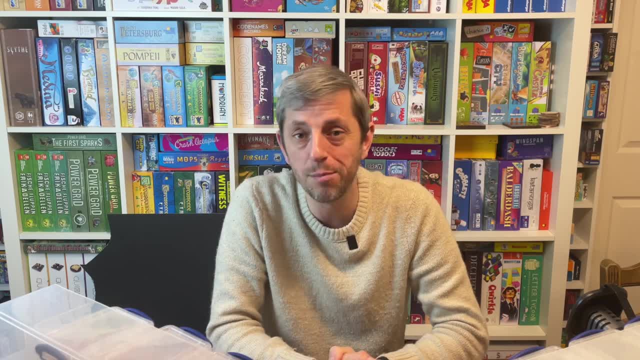 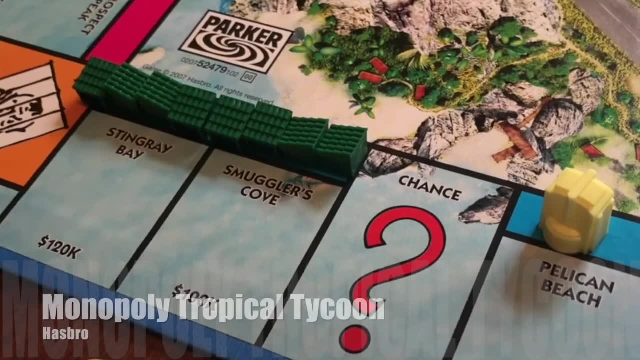 a board game that I love. I've occasionally stripped components out of games that I've discarded. This has generally been where the game has been unsellable and undonatable. I picked up a battered old copy of Monopoly from a charity shop once for the purposes of making a video, and that 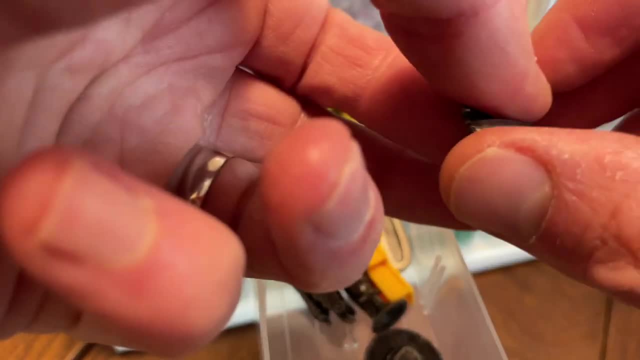 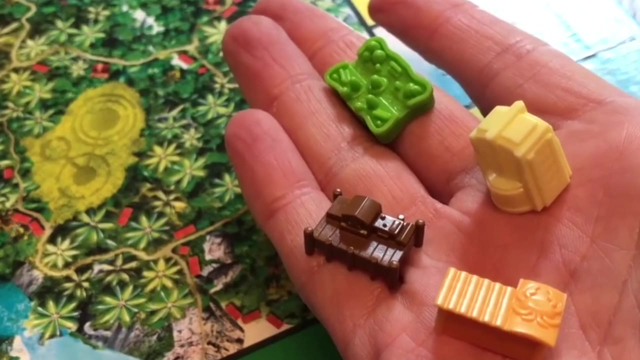 was a good deal. The other components- a metal tank, a sailing boat and a parrot- are lovely but not really of much use because they're unique and I'm always going to need multiples. I had high hopes for a little Japanese game I picked up at Essen called Here Comes the Dog. 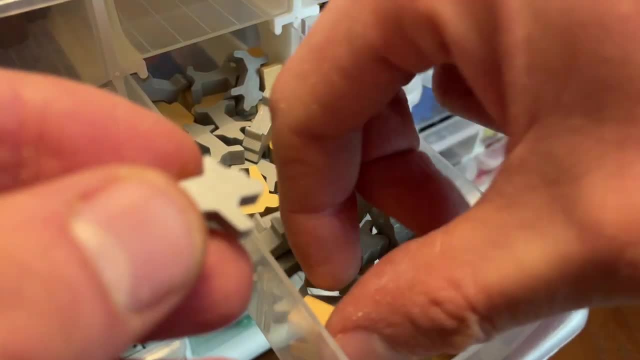 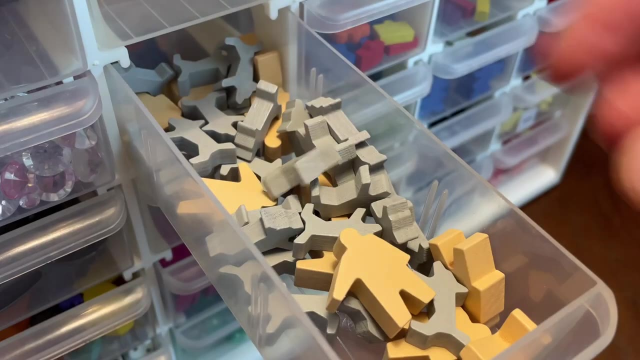 It was pretty much unplayable. Perhaps I misunderstood something, but I didn't want to inflict the game on anyone else, so I ended up with this nice little supply of wooden dogs and their owners. I'm sure I'll think of a game to utilise them one day. 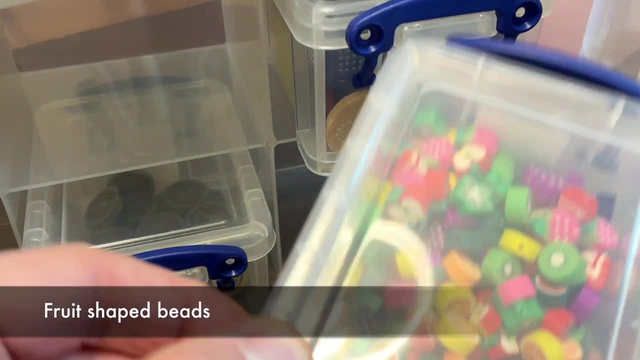 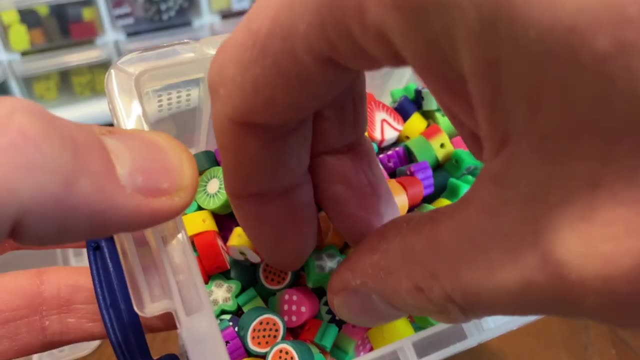 In this drawer I have a nice selection of fruit-shaped beads. I picked them up in a crafting shop super cheap and they'd make excellent components for the right project. Sometimes it's all about being opportunistic, spotting a bargain in an unlikely place. A 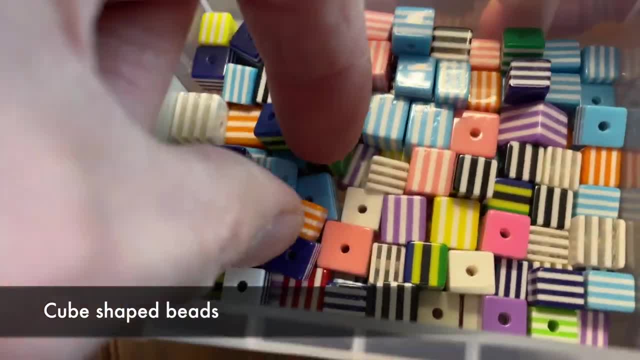 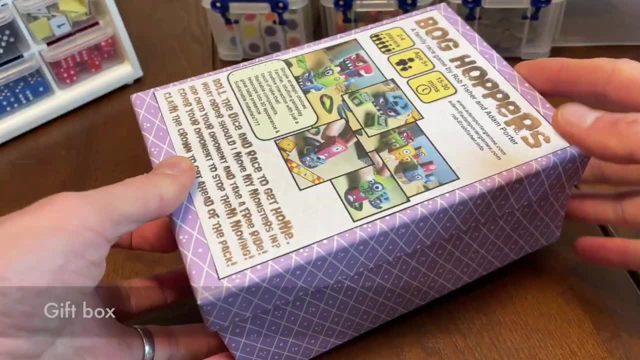 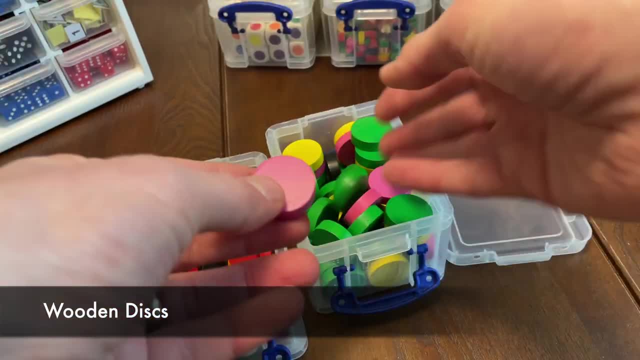 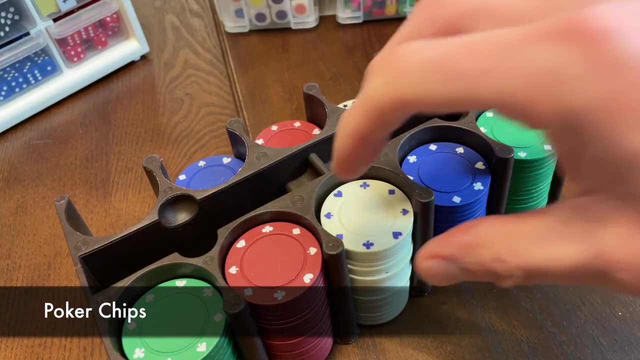 suitcase for trips to Essen. Wooden discs are a similar price to cubes and available from the same websites, but obviously they get more expensive as the size increases. I picked up this set of poker chips from a charity shop for a bargain price and there are enough there to make multiple matching prototypes. 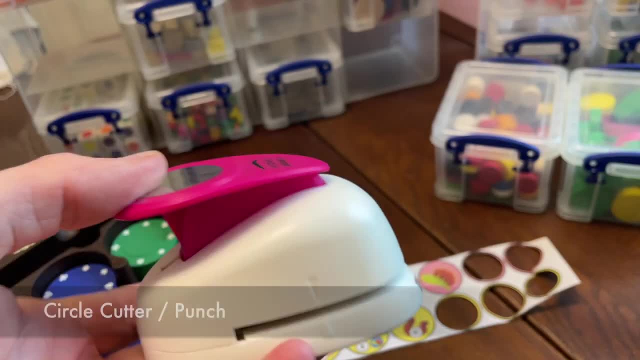 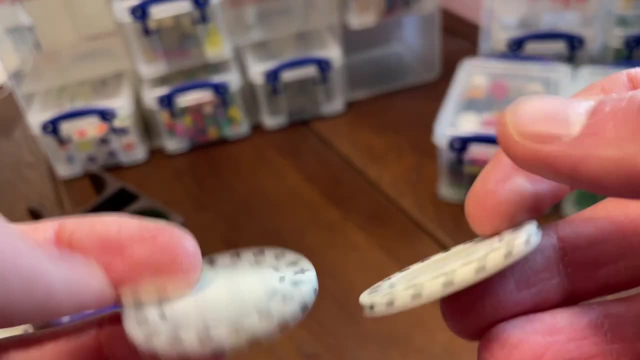 It's really difficult to cut a neat circle to make a label for discs, so I have two circle paper punches at different sizes which do a really nice job of it. Here are some tokens from a prototype battling game that I've been working on. 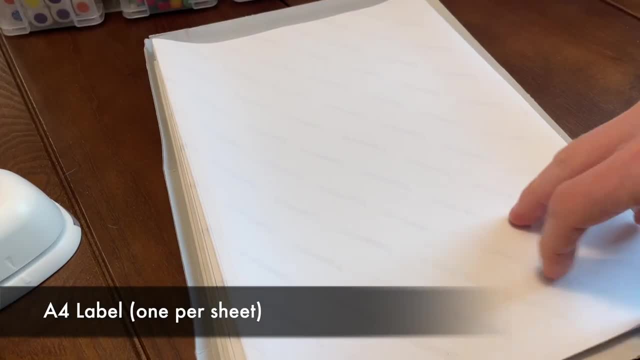 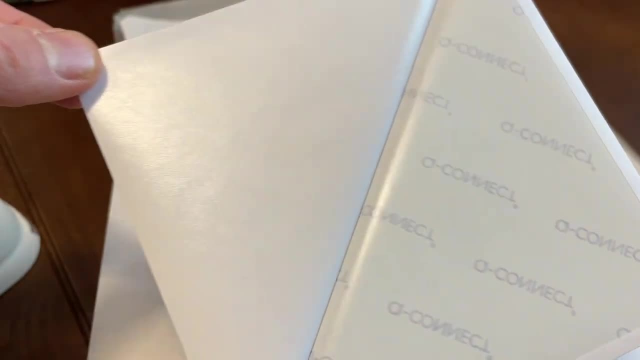 Talking of labels, here's my pick for the most essential piece of prototyping material that every game designer should have access to: A4 labels. One label per sheet. These are easily purchased in any stationery store and they're so incredibly versatile. 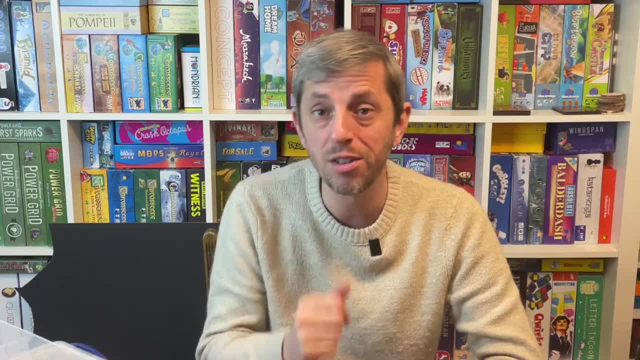 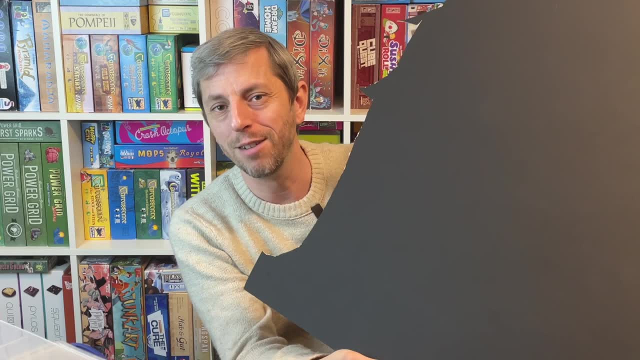 much easier than fiddling around with paper and glue To make tokens. I simply print onto the label sheet. I then use mount board for the token and cut it down to size with a craft knife. Mount board is the thick cardboard used when mounting photographs. 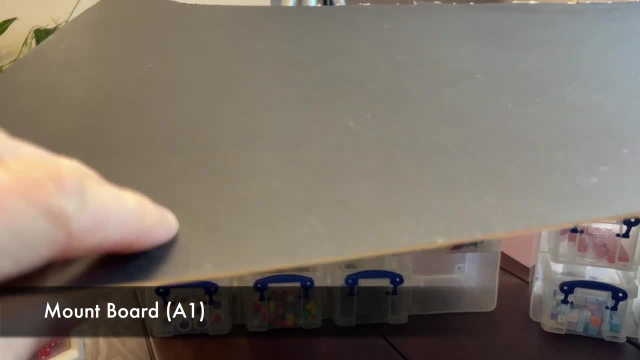 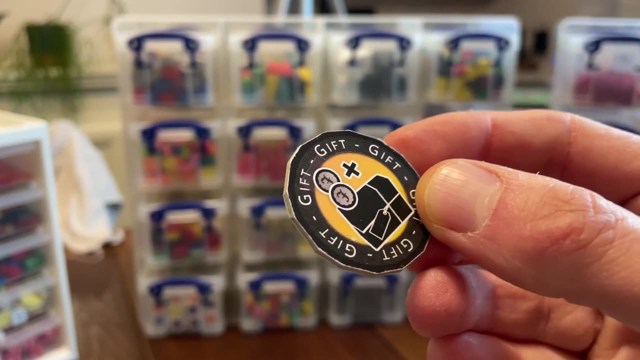 Or paintings. It's just slightly thinner than a carcasson tile and it comes in these A1 sheets. It's hard to cut circular sections of mount board. It's too thick for a circle punch so I tend to cling onto old circular discs from discarded games. 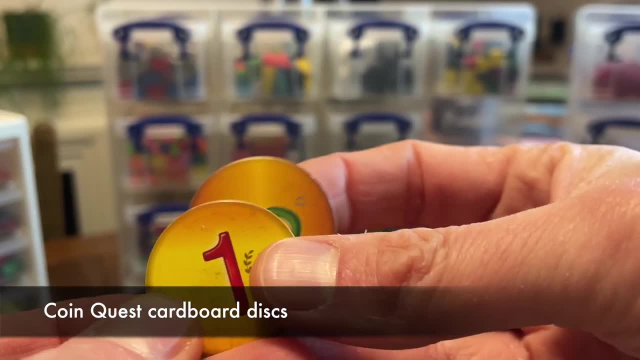 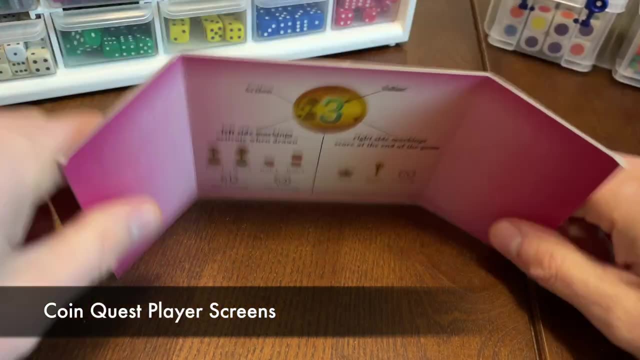 I picked up a game called Coin Quest years ago and had many, many such discs, along with loads of gorgeous felt bags and player screens. I wasn't enamoured with the game, but the components have been really useful for prototyping my games. 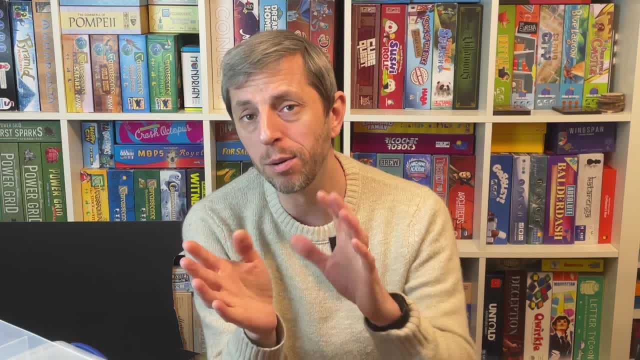 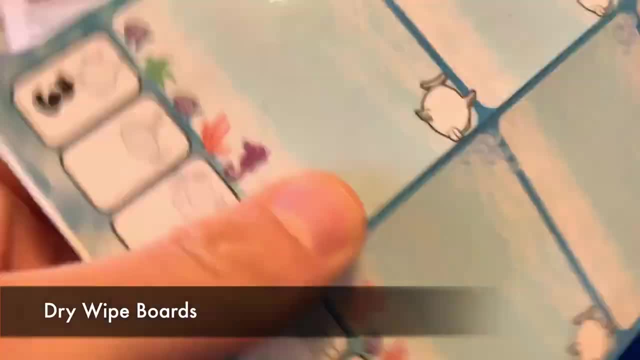 Over the years. Another trick I sometimes use with labels is laminating the sticker sheet after printing on it, but before sticking it to the mount board. I can then peel off the back of the laminated sticker and attach it to the board, creating one matte side and one laminated one. 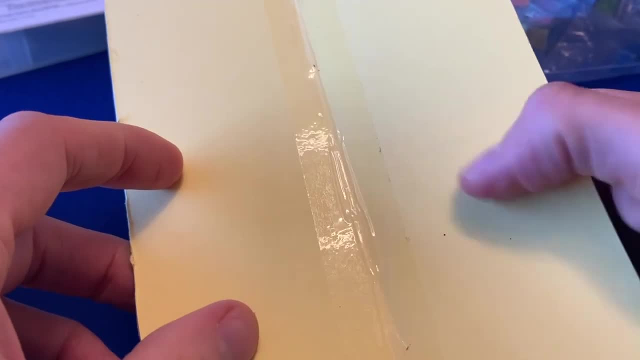 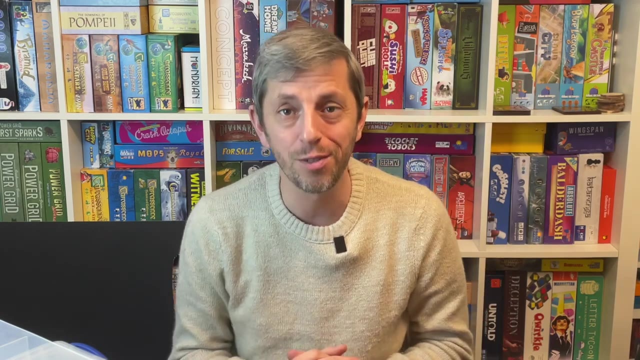 This allows me to write on the board with dry white marker. This was the original prototype for my published game Doodle Rush. Another great thing about mount board is the wide range of colours available. Using different colours is great because you can make tokens with different backs. 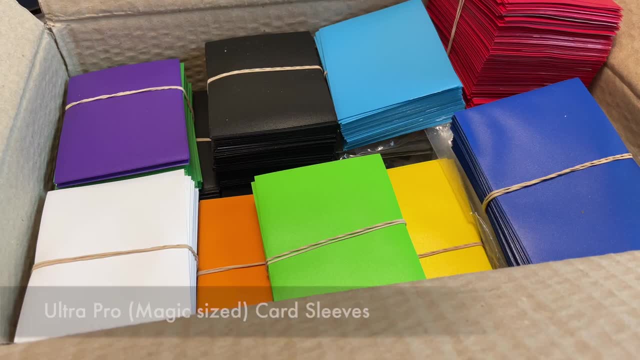 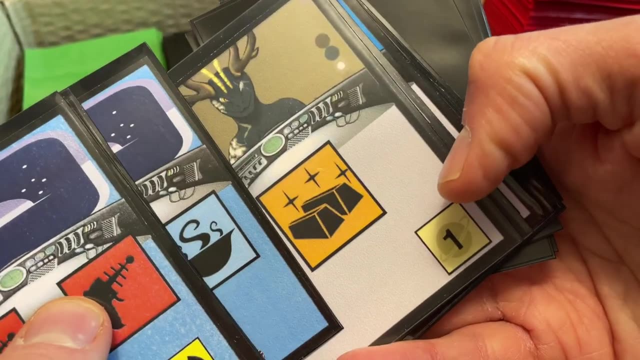 simply by using different coloured sheets of mount board. You can achieve a similar effect with card backs by using coloured sleeves. I tend to print my cards on paper and then slip them into these ultra pro sleeves, which come in loads of different colours. 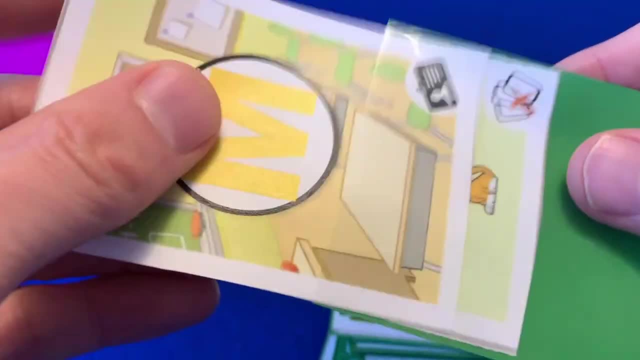 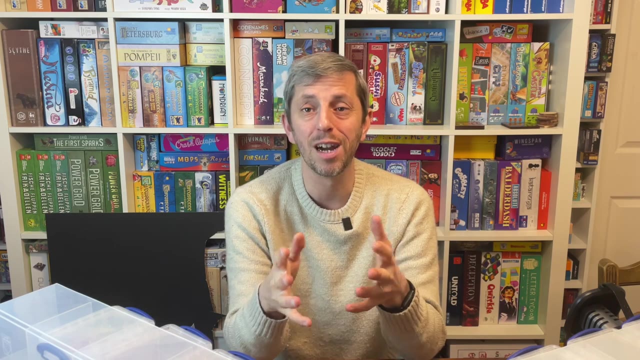 It's a really easy way to distinguish different decks in a game, and a card can easily be altered by removing the slip of paper and replacing it with a new one For a rough and ready prototype, often for the very first playtest, I use blank cards. 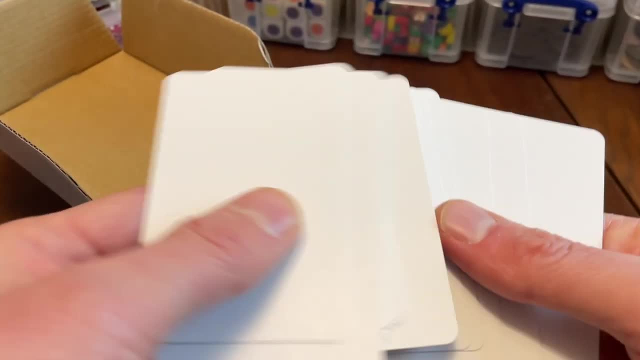 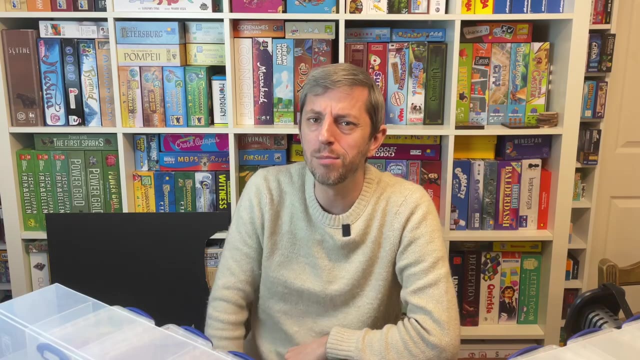 You can buy a box of about 200 for £10, so they're about 5 pence each. Nice and easy to write on quickly with marker pen, and they shuffle well too. Let's take a brief musical intermission and appreciate some of the other components I've picked up over the years. 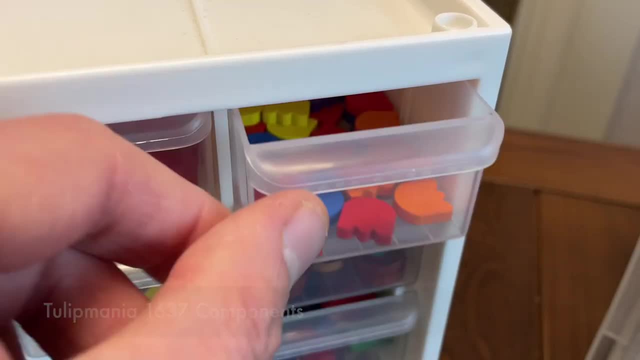 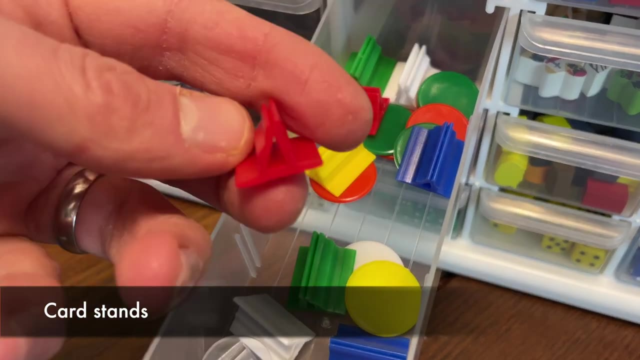 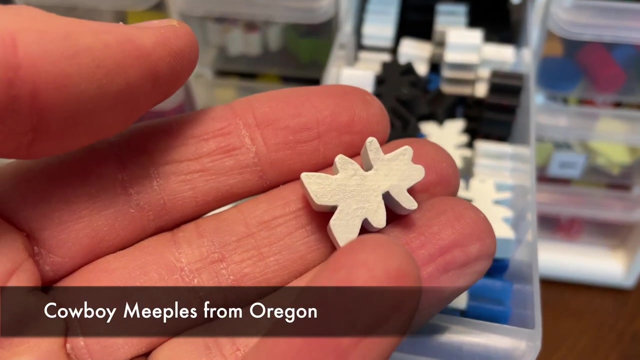 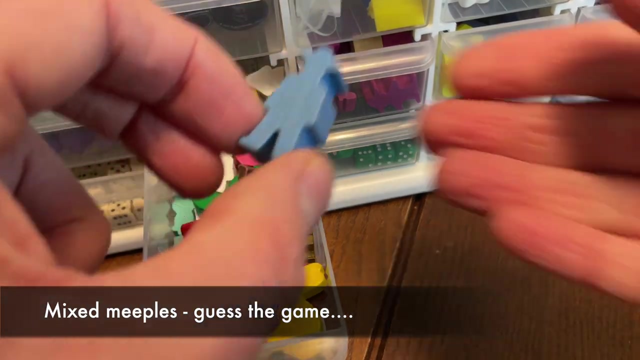 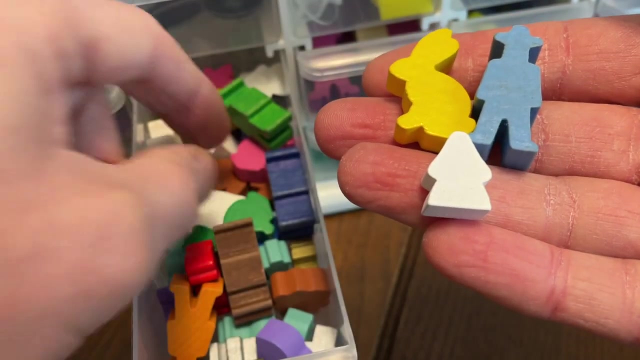 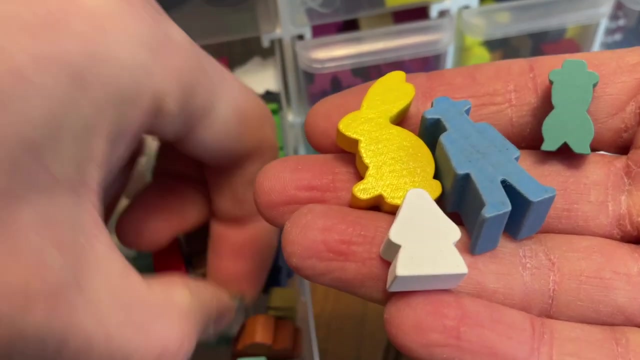 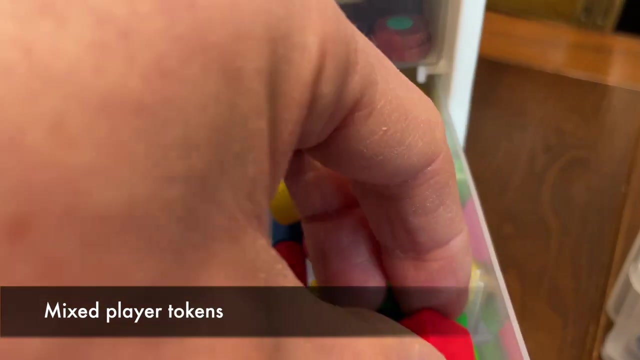 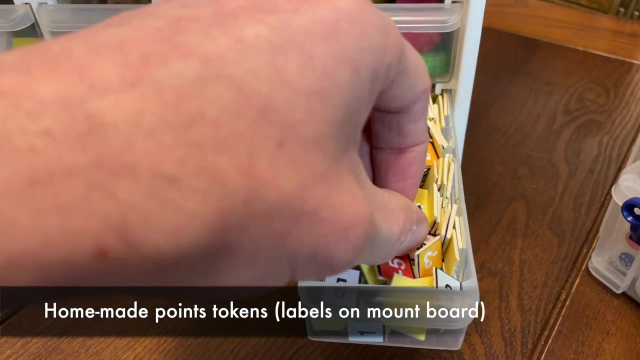 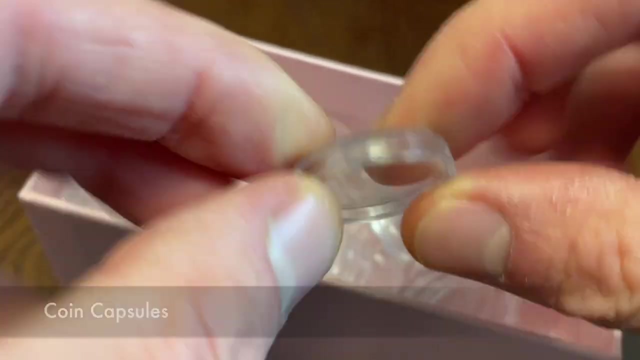 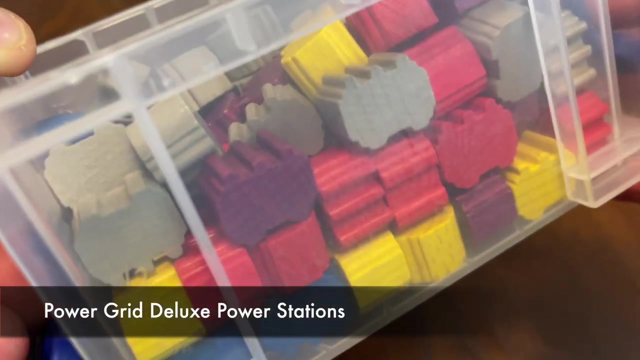 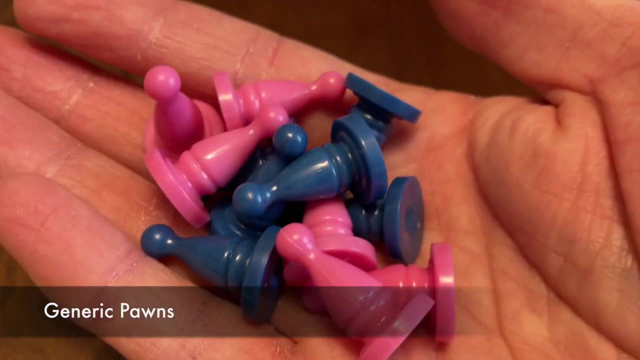 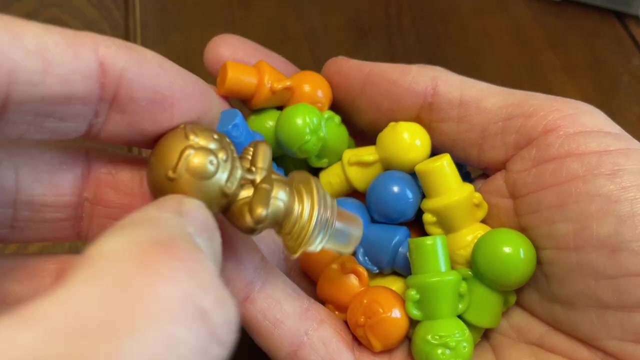 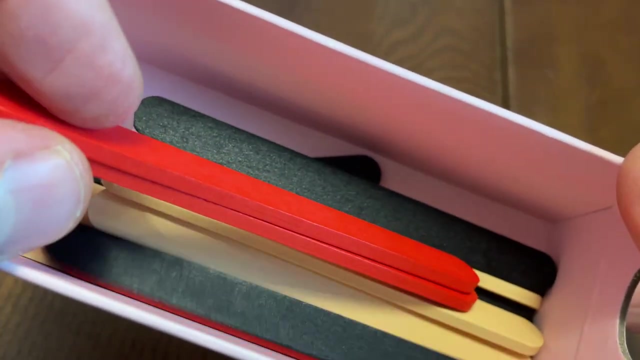 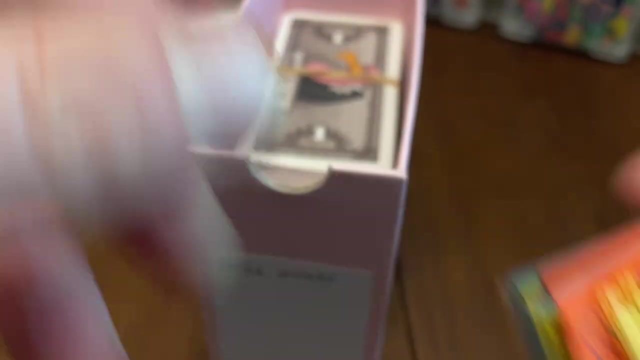 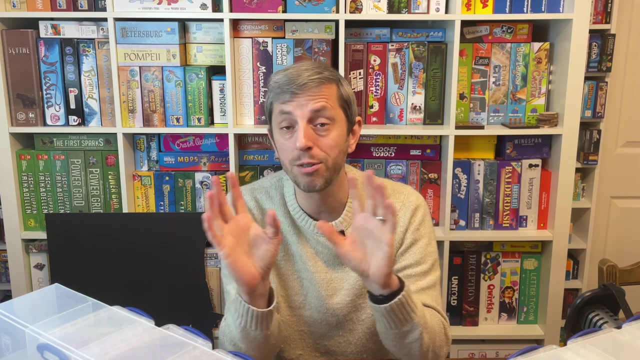 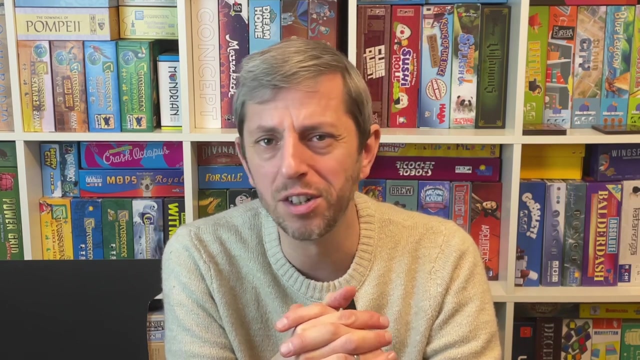 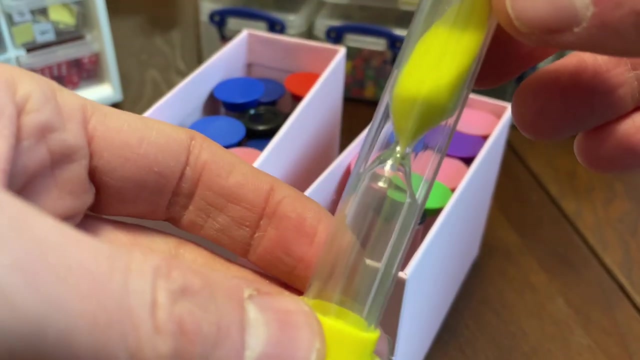 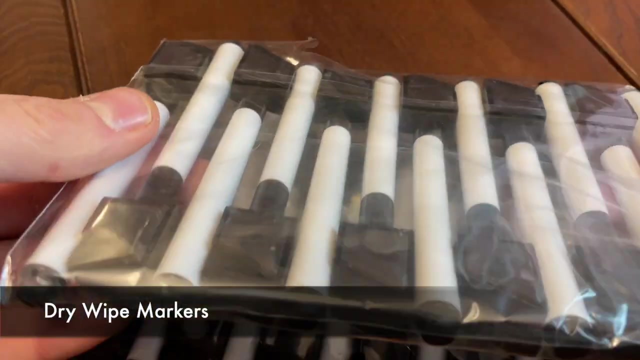 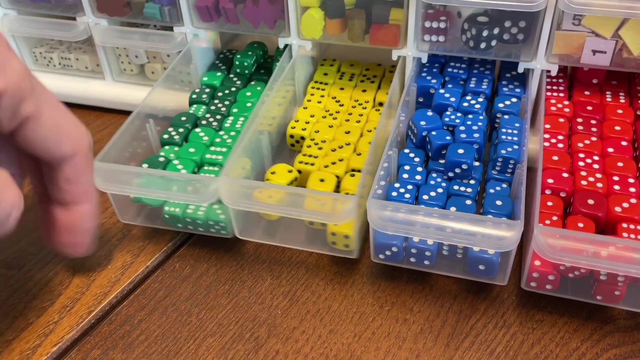 Thank you, Thank you, Thank you. I also have a hefty supply of dry white markers from the same prototypes And, of course, many, many colored dice from my prototypes for Throne, each of which contained 40 dice. 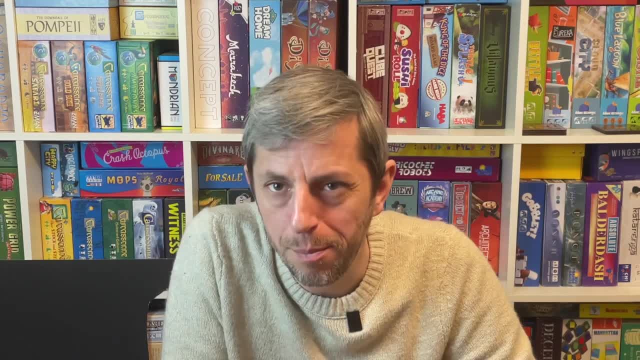 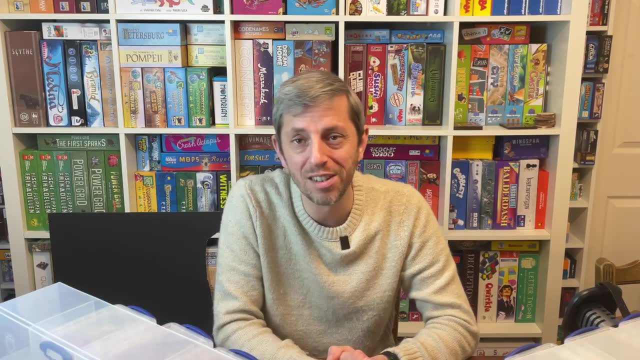 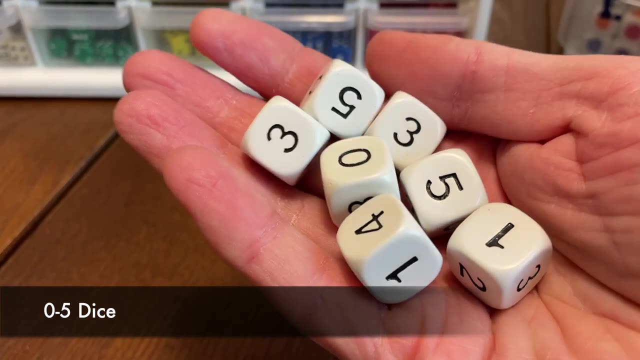 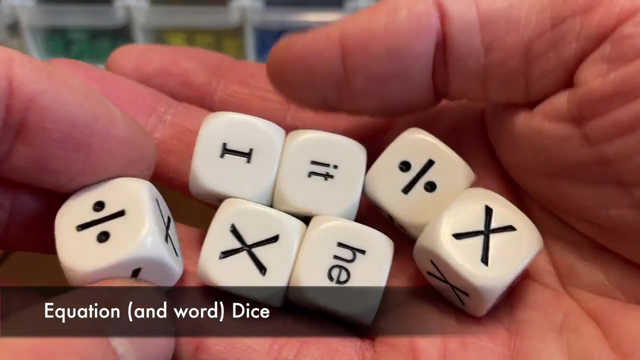 Now, dice aren't cheap, but for prototyping purposes you can scrimp on quality, So most of my Throne prototypes used tiny, tiny dice. Here are some other dice I've utilized in prototypes in the past. If I need custom dice, I always use these blank plastic dice. 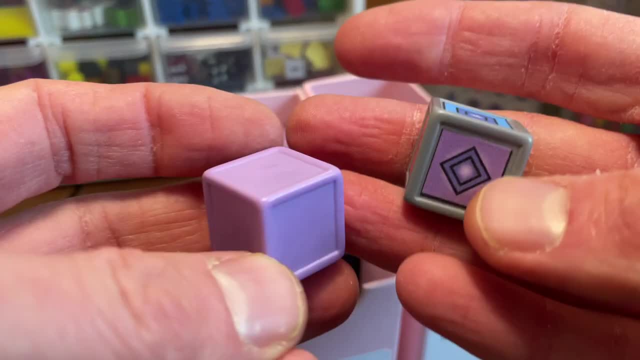 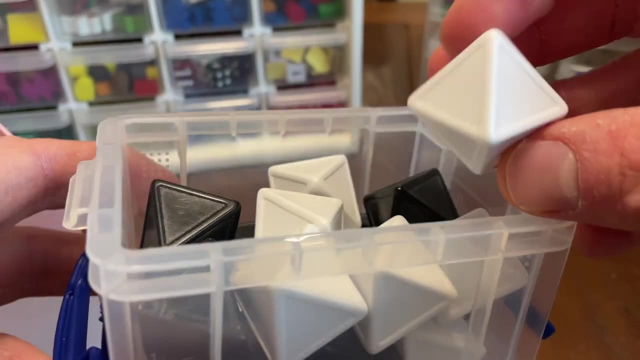 In the UK they're available through an online store called blankdicecouk. You can get them in many colors and even in different shapes. Here are some eight-sided examples. You simply print your labels onto A4 sheets, as I've described previously, and cut and paste. 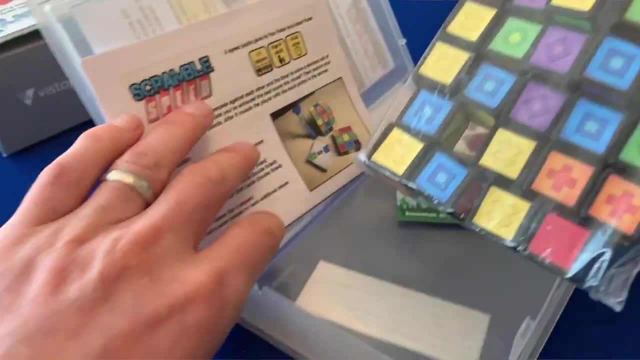 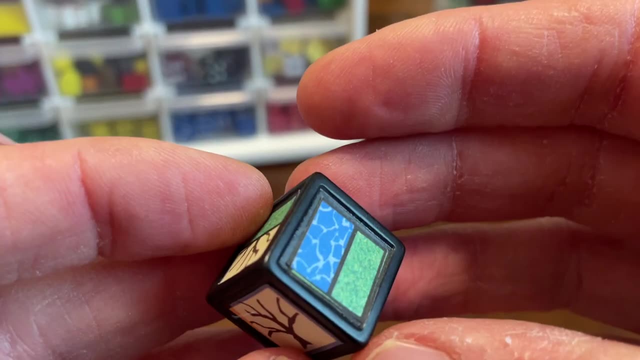 I've used these dice many, many times. I've used them for different prototypes and always have a ready supply, But there's nothing stopping you reusing the dice by simply sticking new labels over the previous ones. This is my fourth organizer and it's a little different to my neat hobby craft examples. 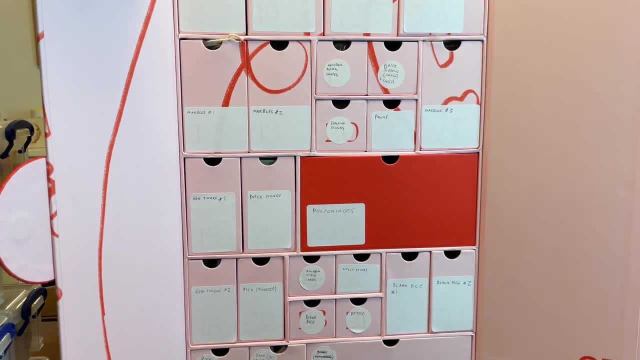 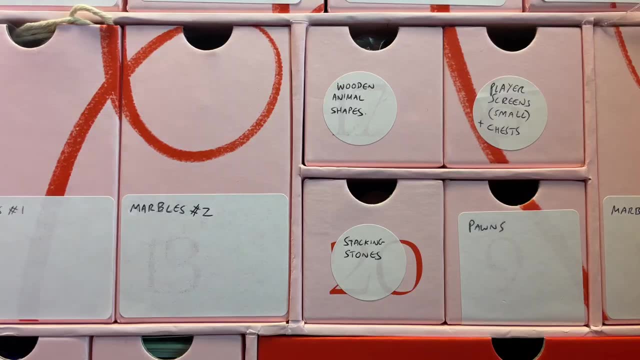 This is an old advent calendar which my wife received one Christmas, full of fancy makeup and perfumes. As any sensible husband would, I spotted an opportunity and repurposed it for storage purposes. This little drawer here has some lovely laser-cut anilines. 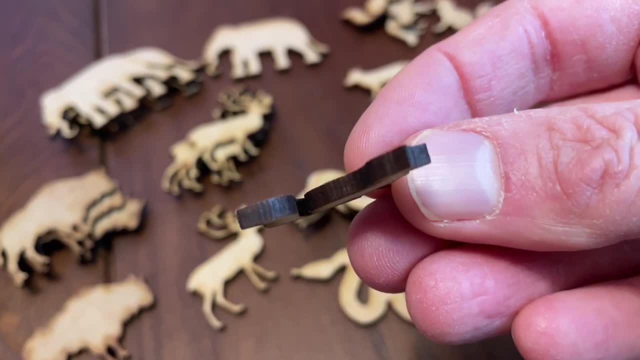 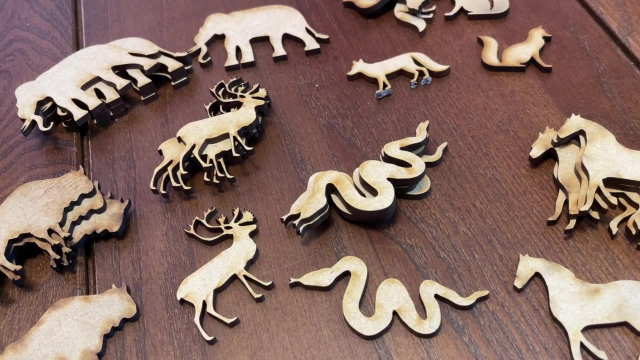 I bought these off eBay with the intention of making an animal-based puzzle game. It didn't work, but I'd love to use these pieces in a later prototype. They came in very affordable little sets. This big drawer has loads of polyomino tiles. 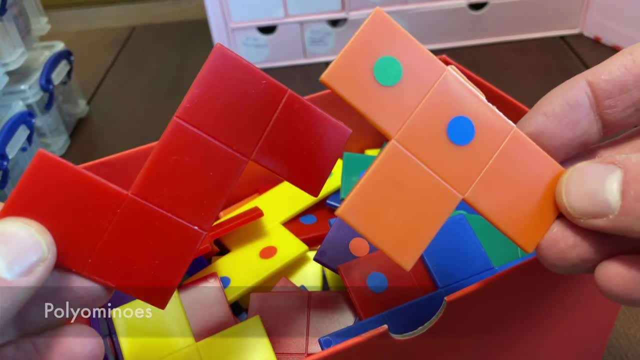 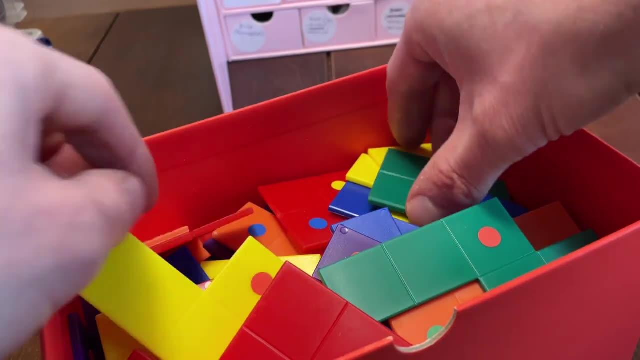 I had the idea of making a polyomino game like Patchwork or Bear and Park, but I dreaded cutting all the shapes out of Mountboard with a knife. So I bought a set of plastic tiles, intended for school geometry lessons, I guess. 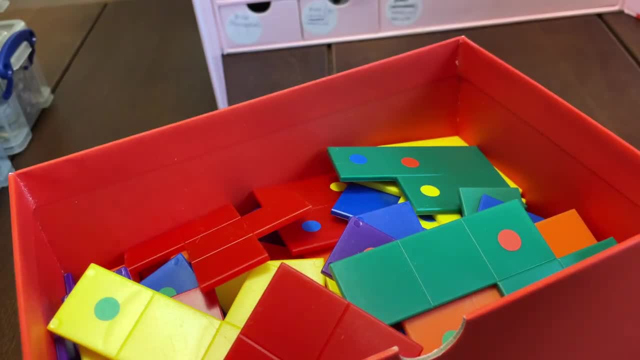 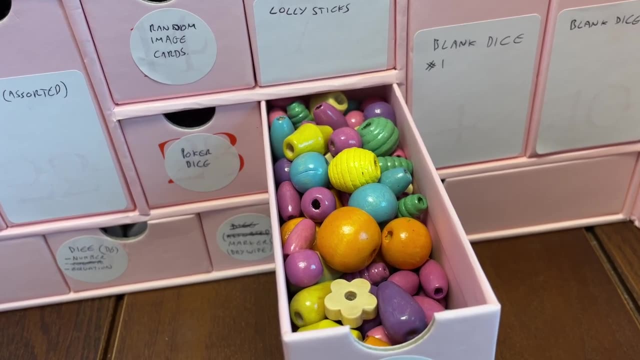 These weren't cheap at all and I don't think they were the right solution. I didn't get far with the prototype. I have sections here for beads, Again picked up cheap from a craft store. Haven't found a use for them yet. 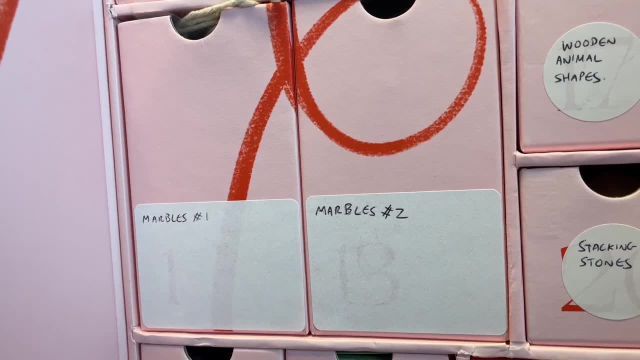 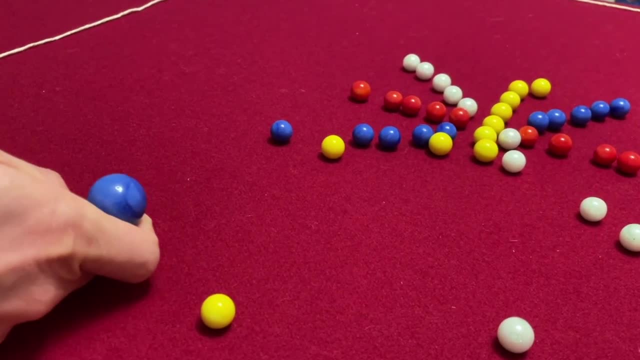 Buttons- which, likewise, I haven't really found a reason to use- And lots of marbles. I really feel there should be more marble-based games. Potion Explosion and Gizmos are holding the fort, But surely there's untapped potential there. 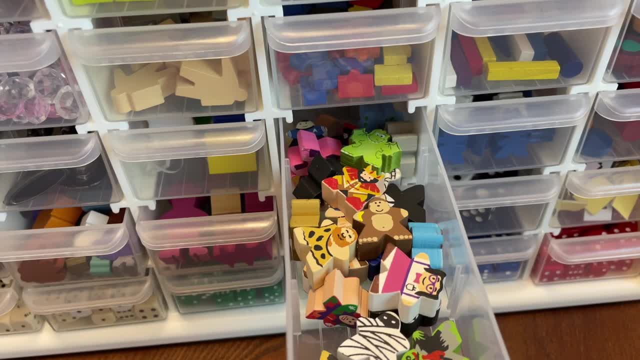 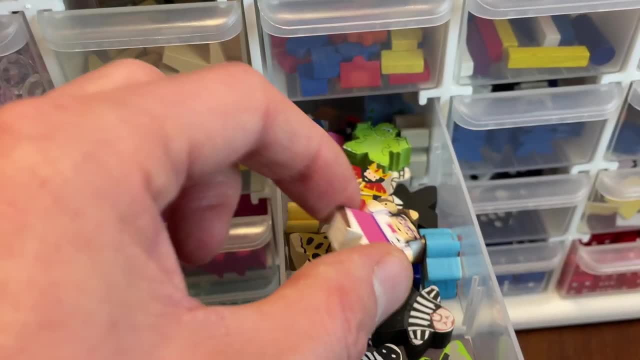 This drawer features an example of how not to do it. In my first ever prototype, I purchased fancy screen printers. I wanted meeples to represent the players and each had their own player power. These were costly to purchase and entirely unnecessary. 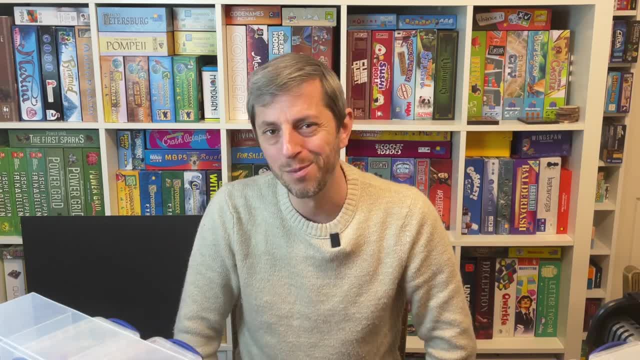 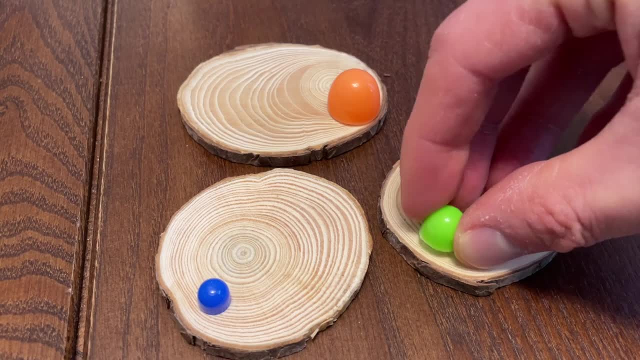 They really could have been represented by plain meeples or even wooden cubes. I recently started experimenting with these little plastic pegs. They can slot into a hole drilled into a wooden block or a piece of foamboard, again purchased from a craft store. 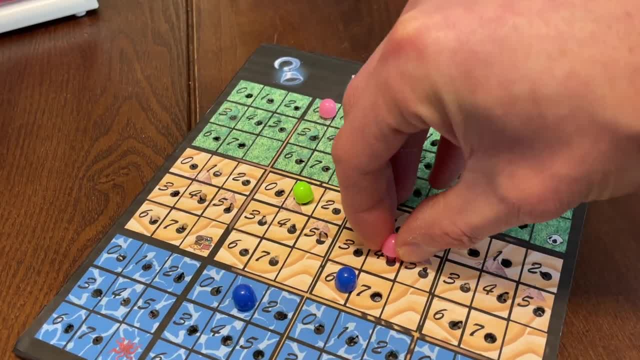 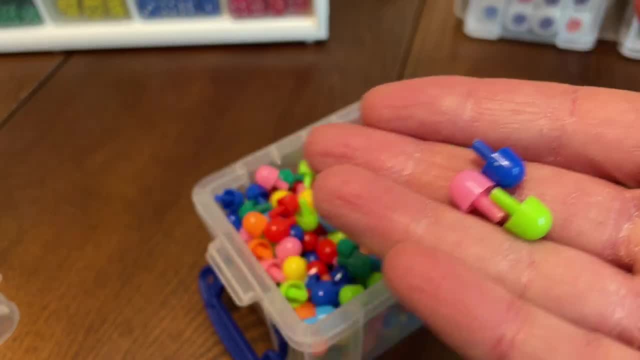 It's really great for a component which isn't going to move. Better than placing a wooden cube, then knocking it off its intended space and not knowing where to return it. You can get these pegs in bulk by buying a children's pegboard craft set. 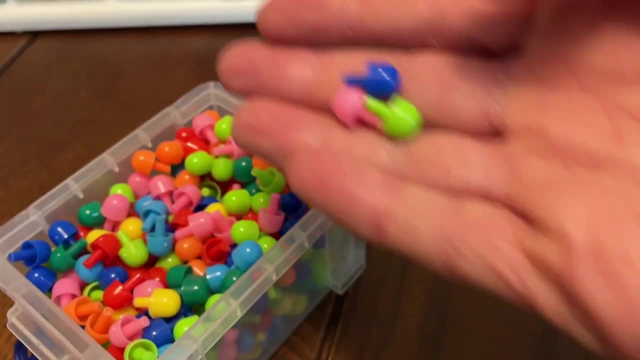 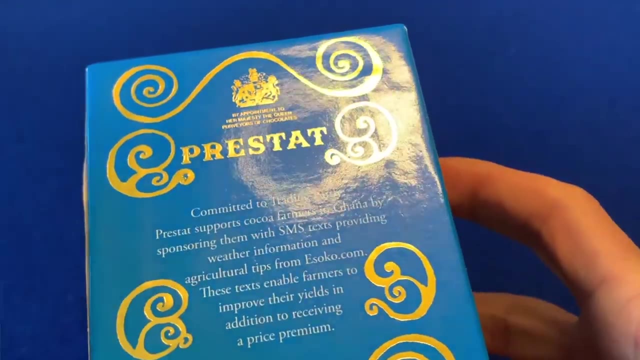 They cost less than two pence per peg. For boxes, I tend to keep anything which is about the right size, of a decent quality and hasn't got too much garish decoration. I love these little Jo Malone perfume boxes which my wife occasionally picks up. 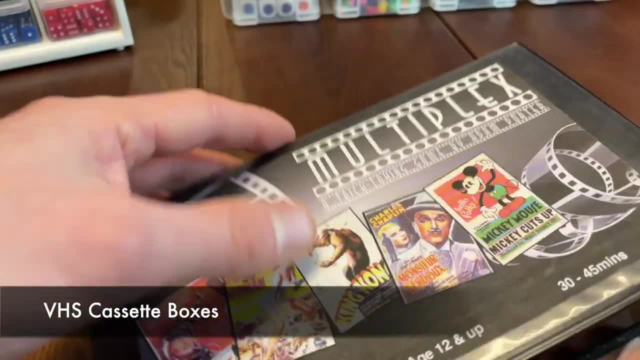 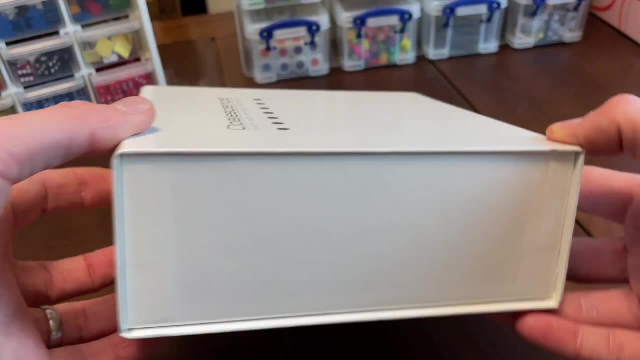 Great for little card games. VHS video cassette cases are also good for card or dice games, And these magnetized boxes which I got from work are just perfect for a slightly larger game. They originally contained tooth whitening kits. I'm a dentist. 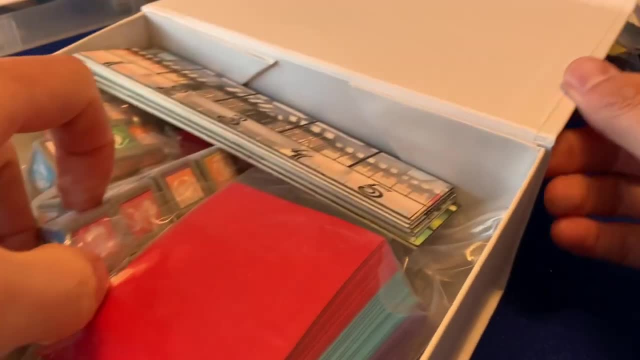 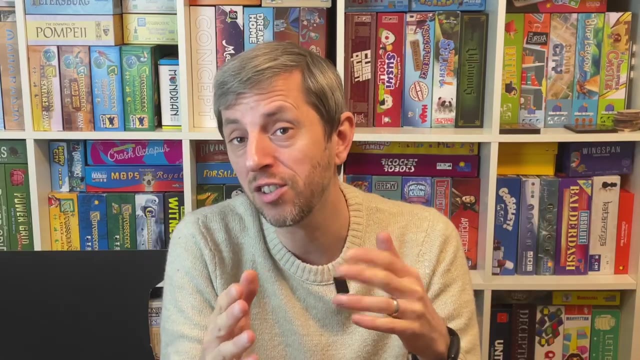 But I love how plain they are. I can simply stick a label over the branding and it's a perfect little package. I recently had a real packaging dilemma. Perhaps you can help me. My game involves flicking discs across a board and I want to create a prototype. 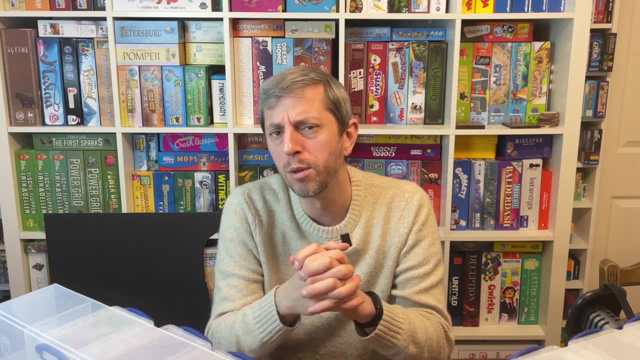 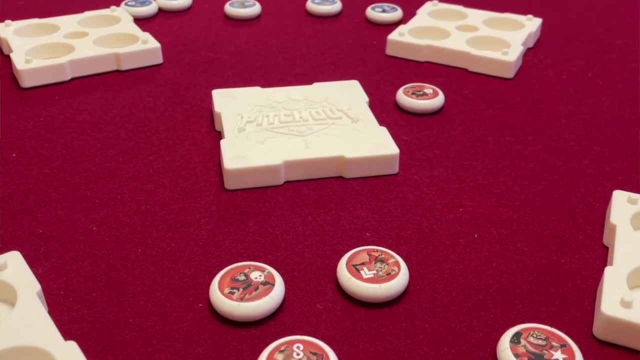 with a smooth surface to flick on which can be shrunk down to fit into a portable box to transport to trade fairs. Looking at comparable games, this one out has no board at all. It simply uses the tabletop as the board. This doesn't work for my game. 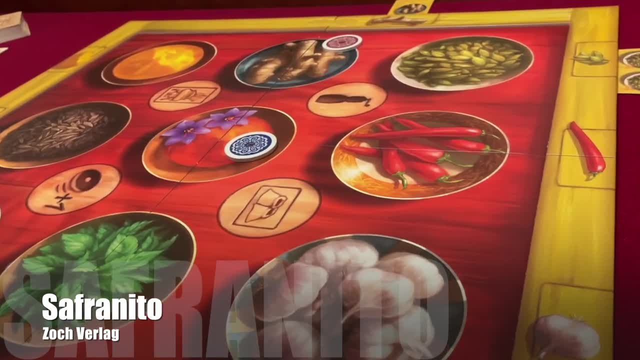 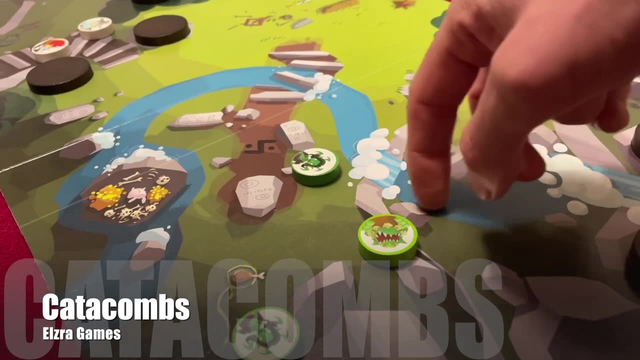 because certain areas need to be marked. Saffronito and Catacombs both feature folding boards and they're beveled so that the crease doesn't interfere with the movement of the discs. I've found this impossible to replicate in a homemade prototype using folded mountboard. 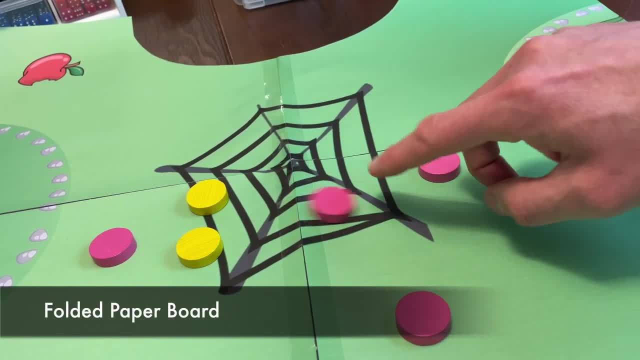 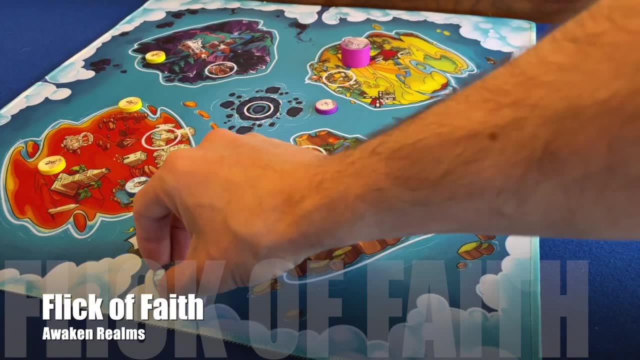 ordinary cardboard or even paper. A crease always interferes. The third alternative is to use a system-like flick of faiths to fold up neoprene mat. Now, custom-printed neoprene is too expensive to use in multiple prototypes. 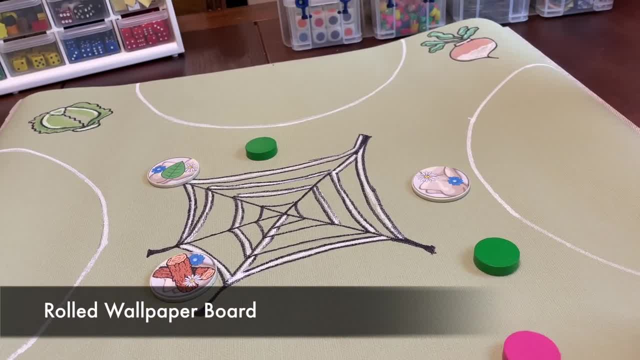 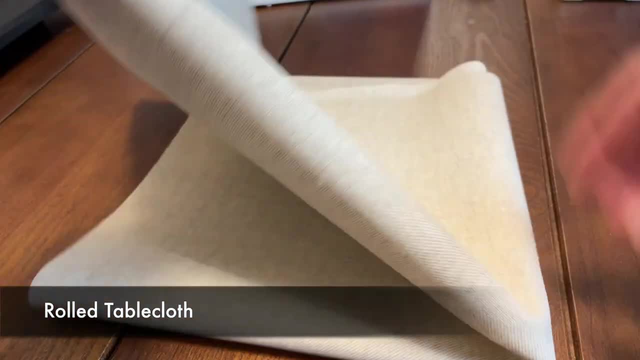 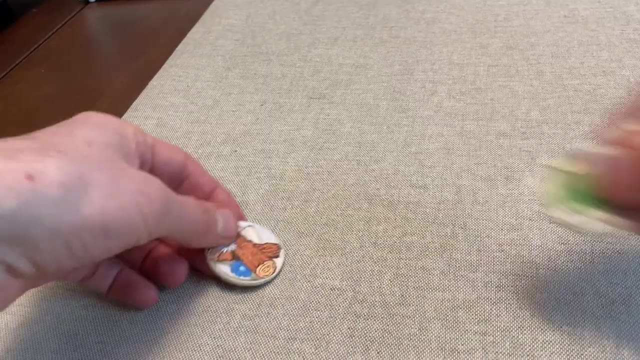 so I've opted to use wallpaper, which is cheap, rolls up well but is of a good thickness. An alternative approach was to use a cheap wipeable tablecloth material. I was hoping this would fold without leaving creases, but it doesn't really work. 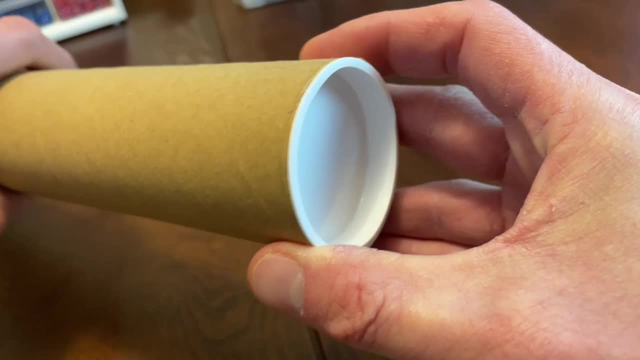 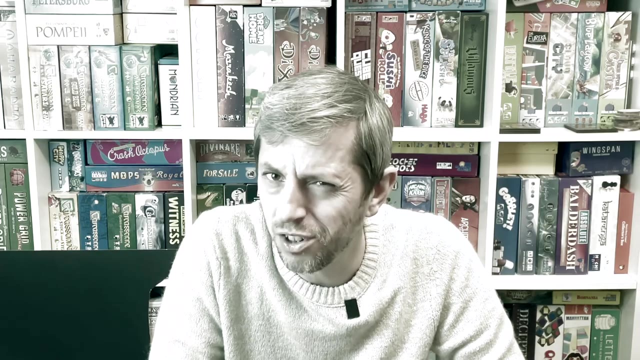 so it still needs to be rolled. The problem is that this means the mat still needs to be blue-tacked to the tabletop to keep it flat. Are there any better solutions that I'm missing? Well, there's a neat little demonstration that board game design isn't all about.